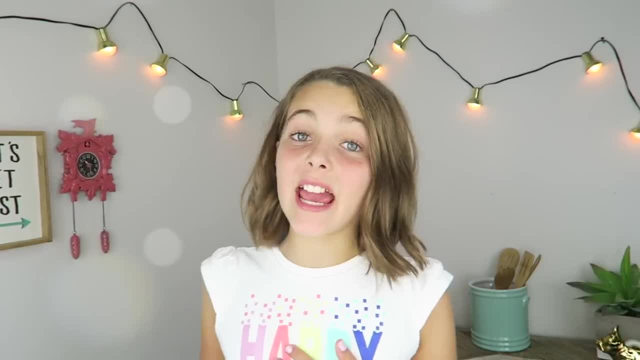 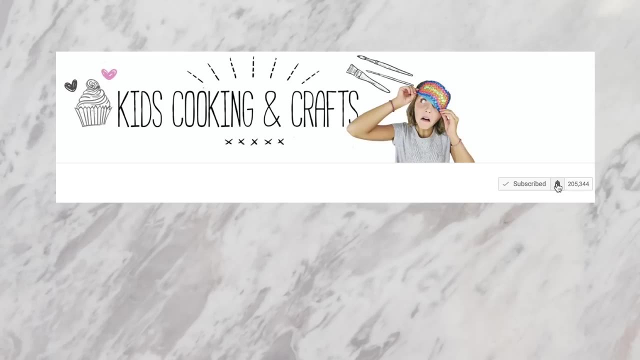 Hello everybody, welcome back to Kids Cooking Crafts. I'm Ava and today I'll be showing you how to make a fluffy slime princess dress. Before we get started, don't forget to subscribe and hit that little notification bell so you know when we upload a new video. 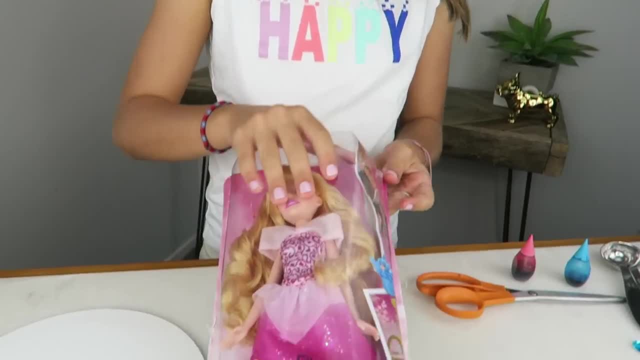 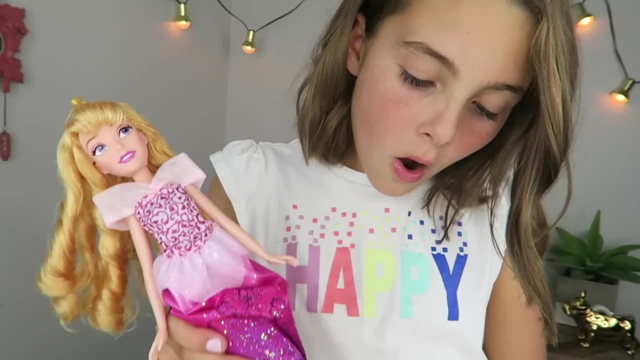 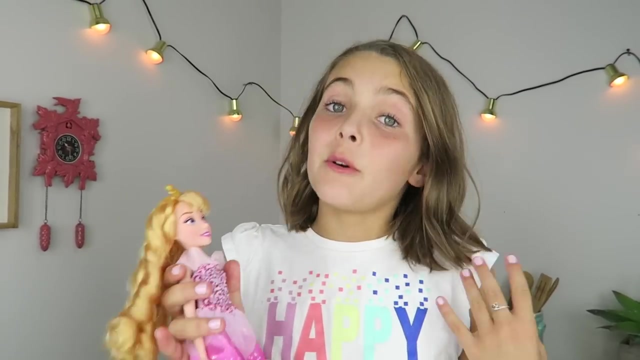 Okay, let's open this package up. Ooh, I love her hair. It's so bouncy. Look at these shoes. Okay, I figured out a way to make her stand up. This is what we're gonna do. First you need a paper towel roll, and then you need a circle piece of cardboard. 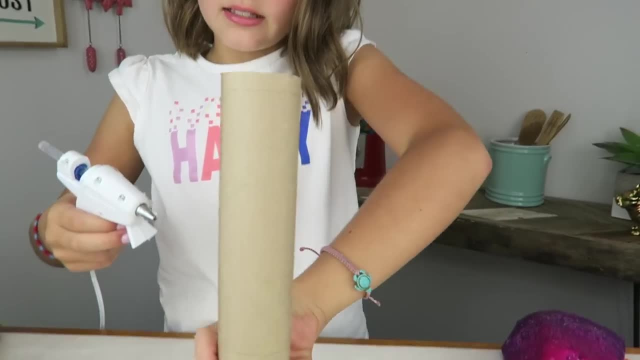 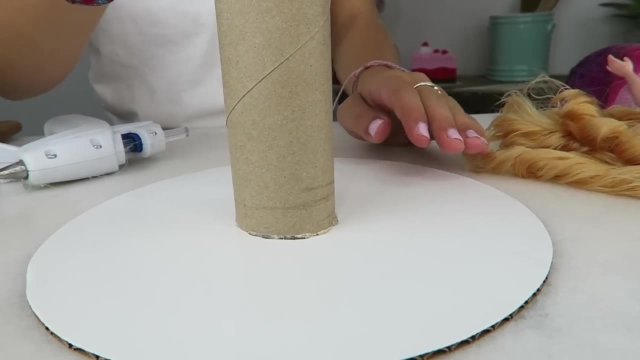 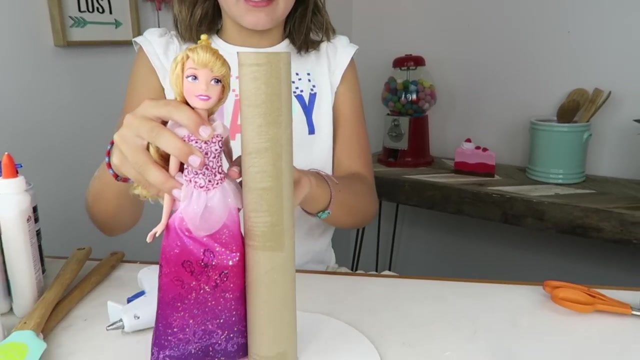 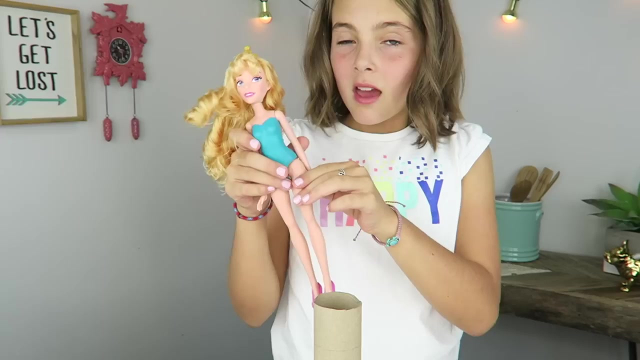 Now let's just put hot glue around it and then stick it on right there. See, look, Now it will stick. We're gonna cut the tube the length of her legs. I'm gonna mark it right where her hips are. Alright, now let's put her in. 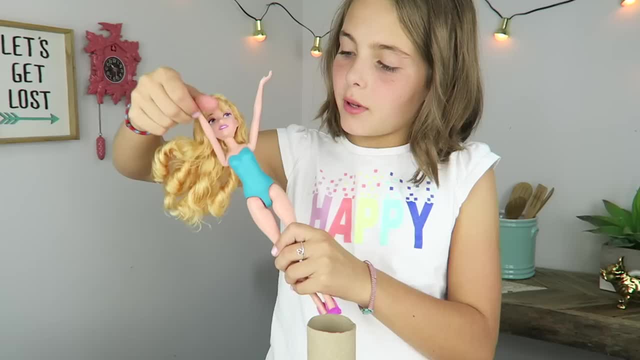 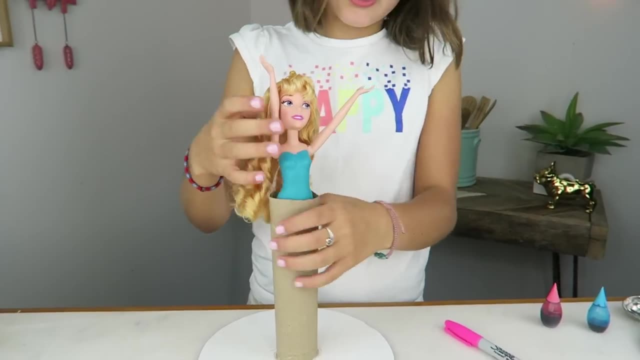 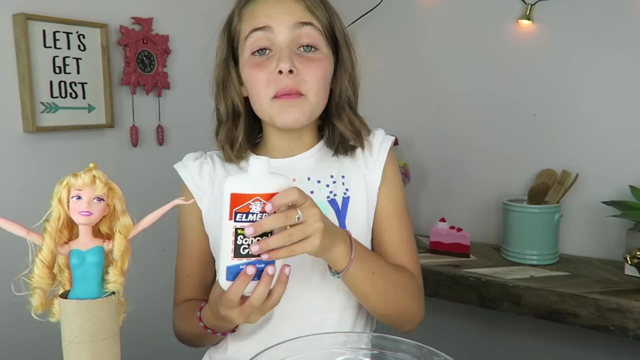 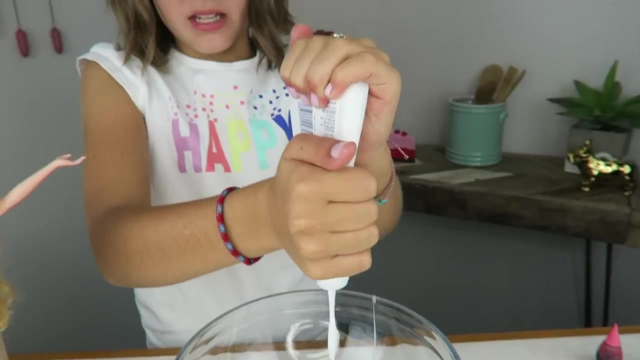 Make sure to stick her arms up There. Now she's gonna stand up. Yay, Alright, let's move this aside and start making our slime. One bottle of glue going in. Oh, that was a big bubble. Alright, now comes my favorite part. 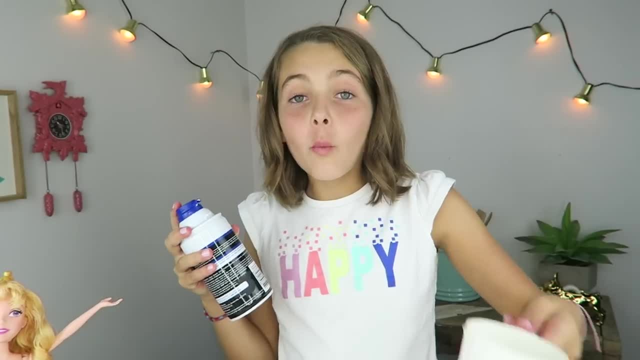 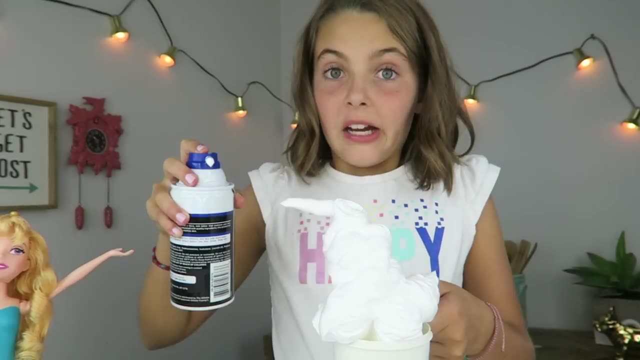 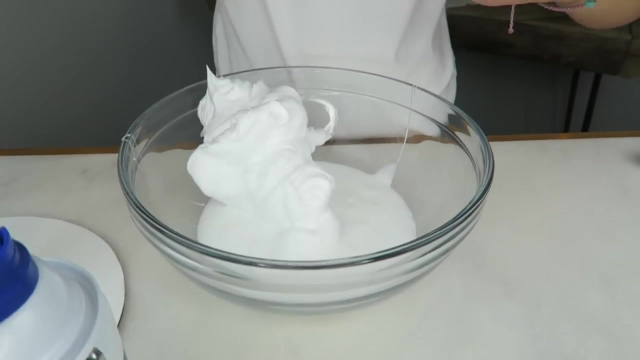 The shaving cream. You're gonna want one cup of shaving cream. Uh, maybe that was more than one cup, but that's okay. We want it to be fluffy. Now let's stir it. Okay, let's add some food coloring. 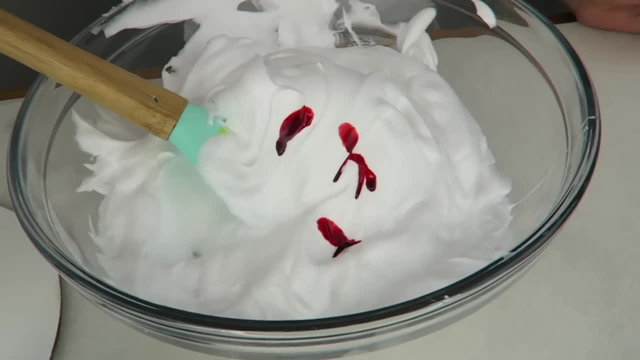 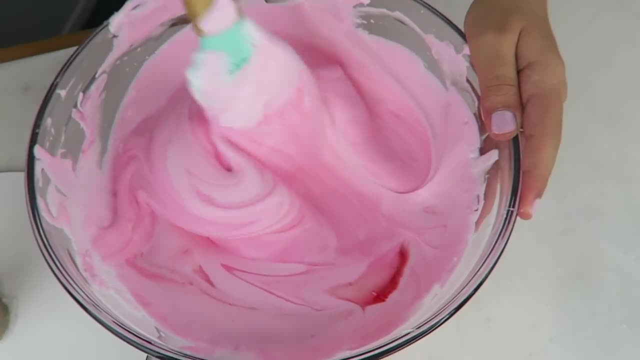 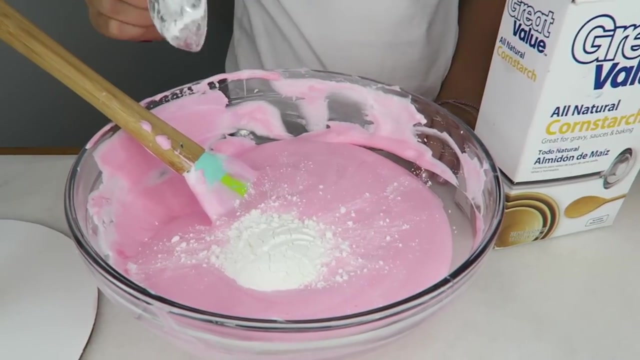 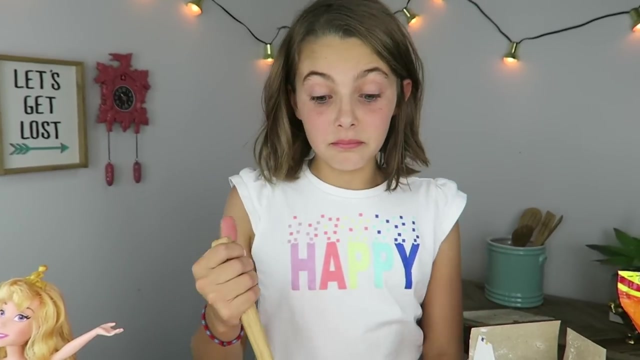 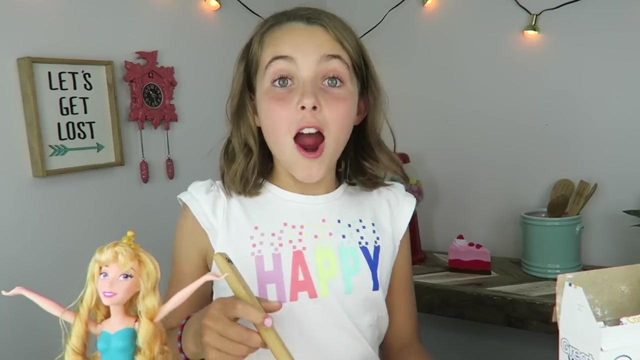 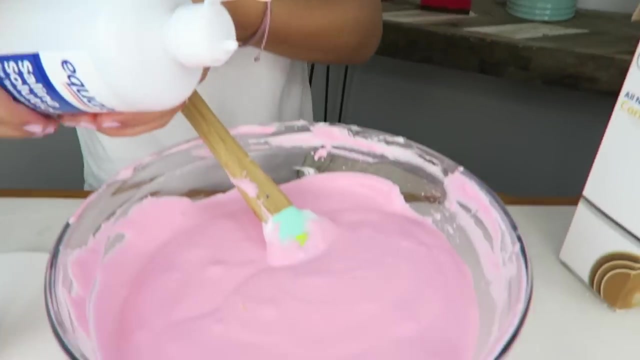 I think I'm gonna do pink first. So next you need one tablespoon of cornstarch, And then you need one teaspoon of baking soda. Now you just stir it up, Alright, next step: You need contact solution. We're just gonna give it a couple of squirts. 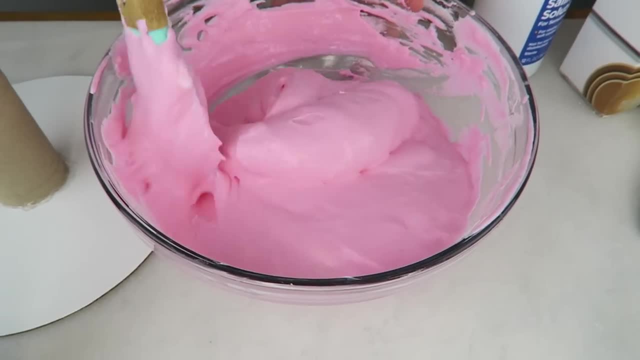 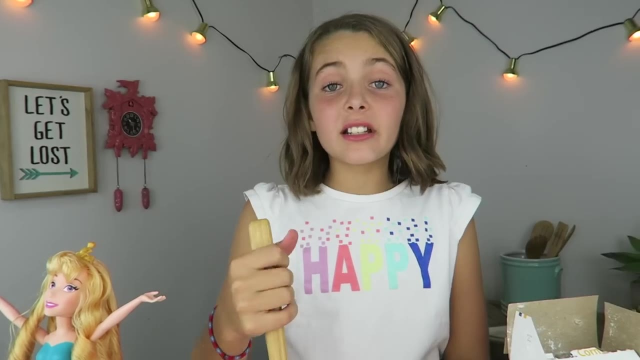 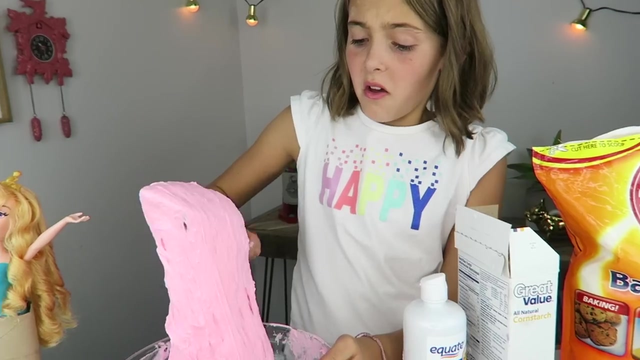 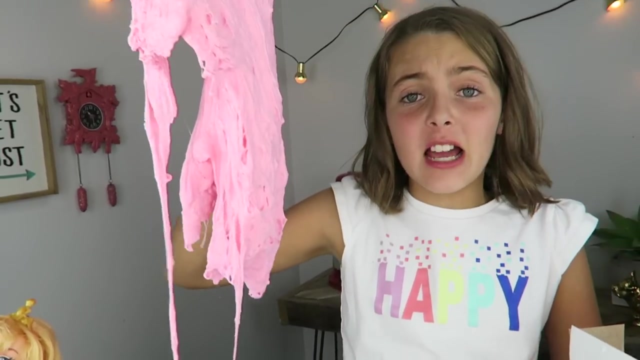 There Now stir it up. Oh yeah, now it's starting to look like slime. Stir it a little bit more, then I'm gonna start using my hands. Oh, this is getting tough. I think it's about time to use my hands. 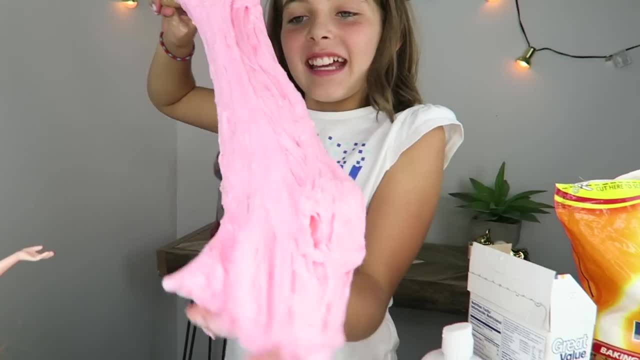 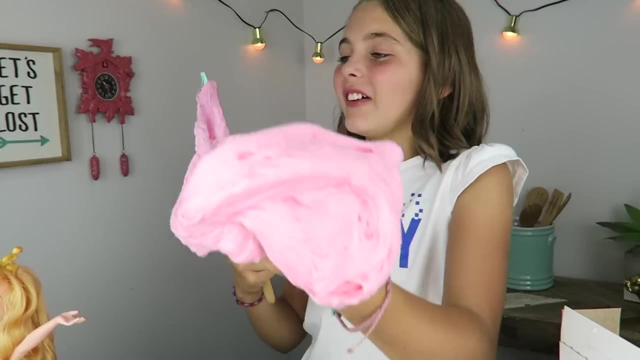 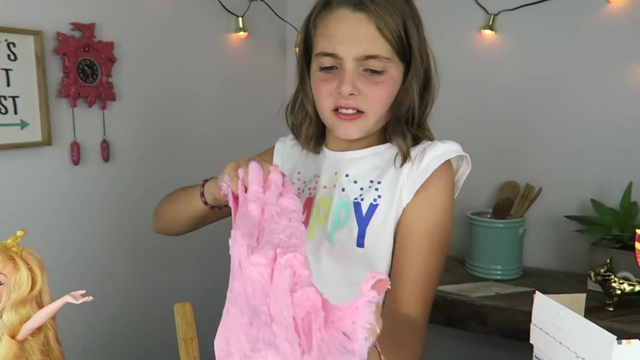 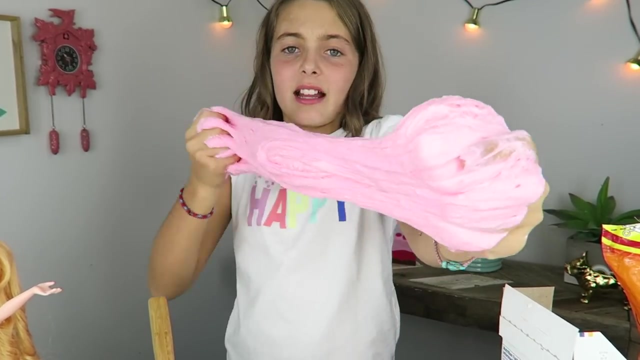 Ewww, Ewww, this feels so weird. Ewww, Okay, this Alright, now you just wanna start Smooshing And stretching, Smooshing and stretching, And keep on doing that until it makes slime. 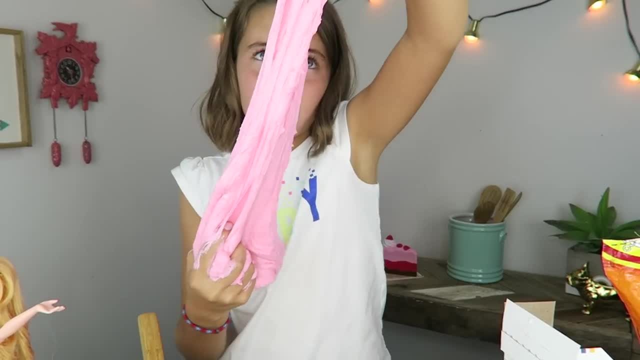 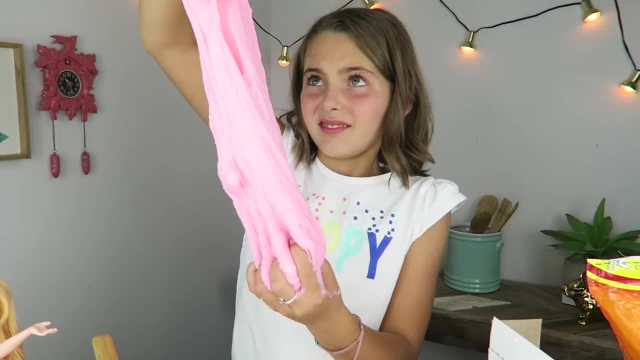 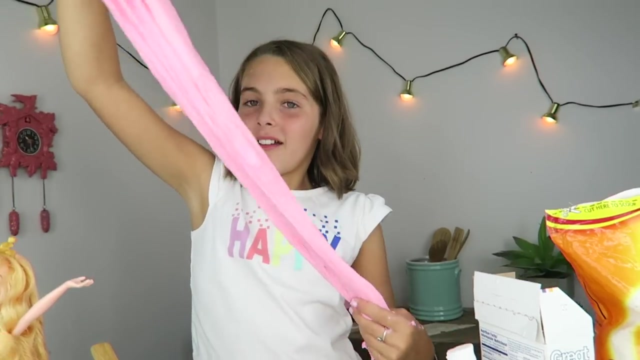 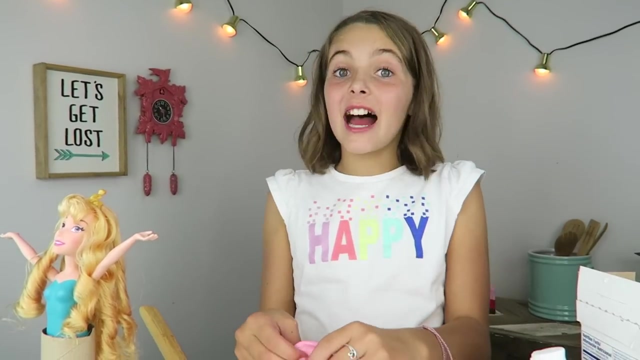 When you know it's ready, it will start coming off your hands. Whew, this is a workout. Whoa, This is awesome. I love this recipe. Now let's start making another batch, But this time we're gonna do blue. 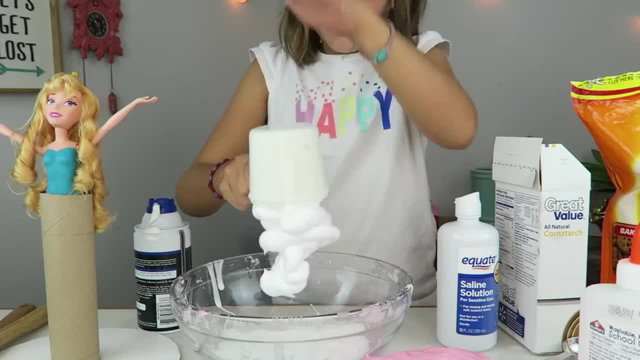 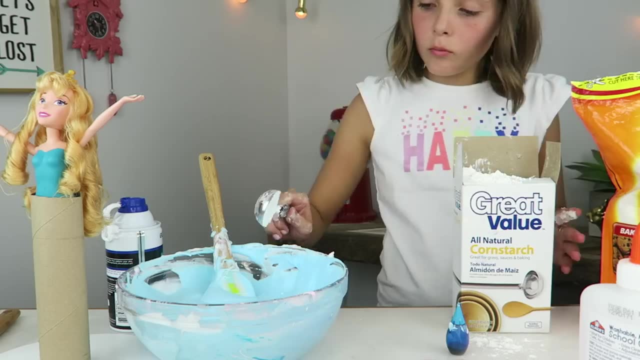 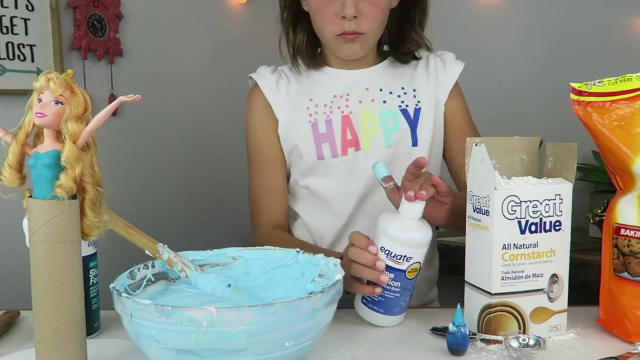 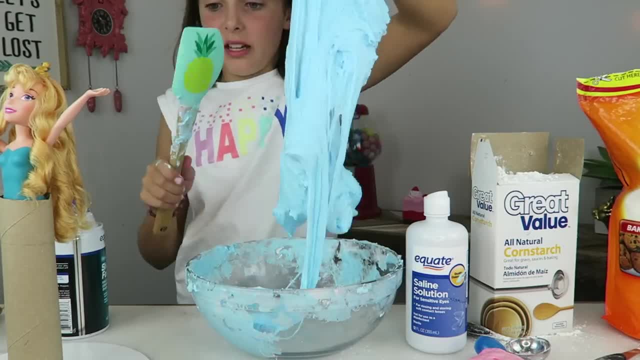 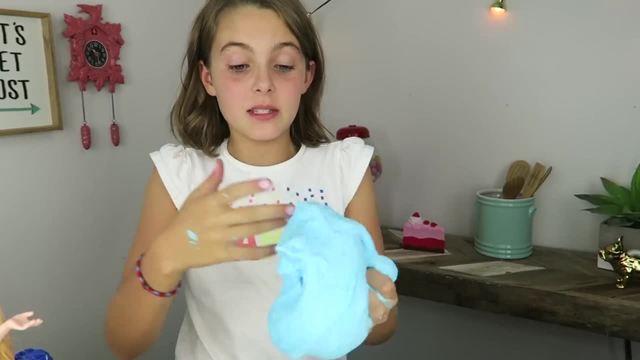 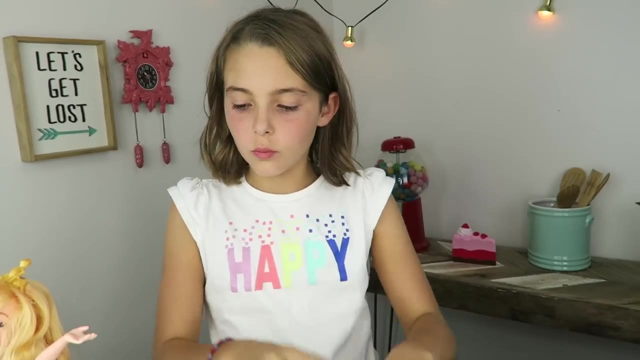 Smooshing, Smooshing. Oh yeah, I think these slimes are ready. Time to make our fluffy, slime princess dress Woo. First, we need to put a ponytail in her hair so it doesn't get slime in it. 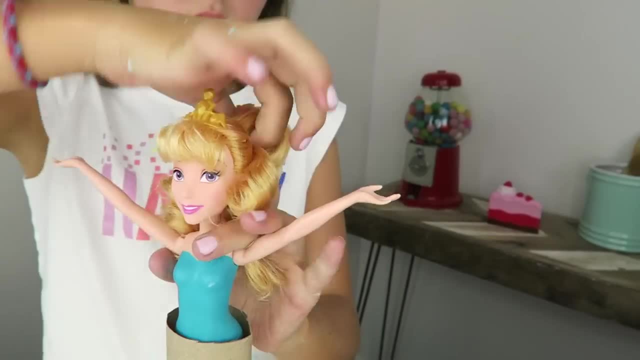 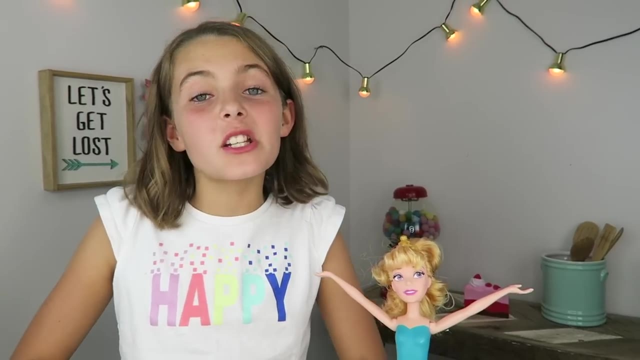 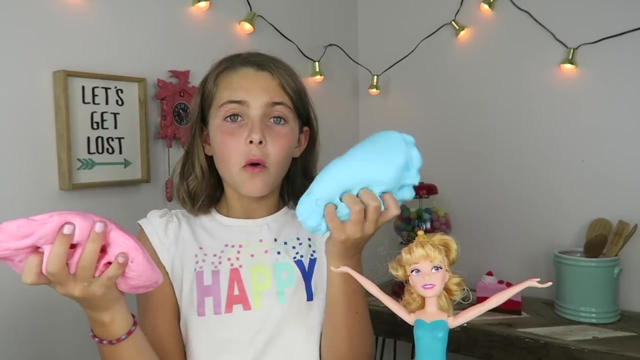 Ugh, that would be the worst. There. She looks so pretty, So in the movie with Sleeping Beauty, when she's dancing with the prince, the fairy godmothers are like: what dress should we make? A pink or a blue? 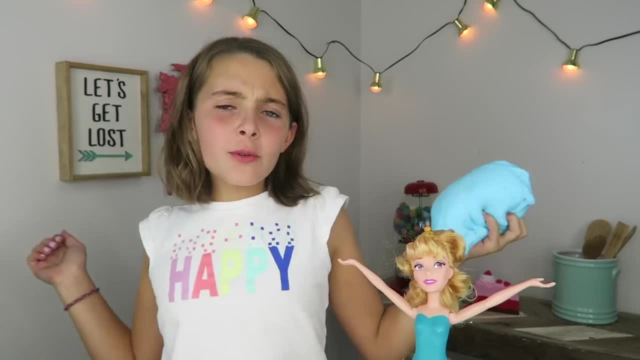 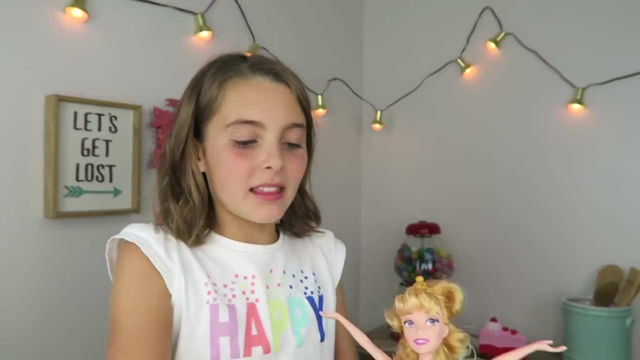 We can't decide And they're like pink, no blue, no pink, no, blue, no pink. So I decided I'm going to do both. I'm going to make this side blue and this side pink, And I may even mix them together later. 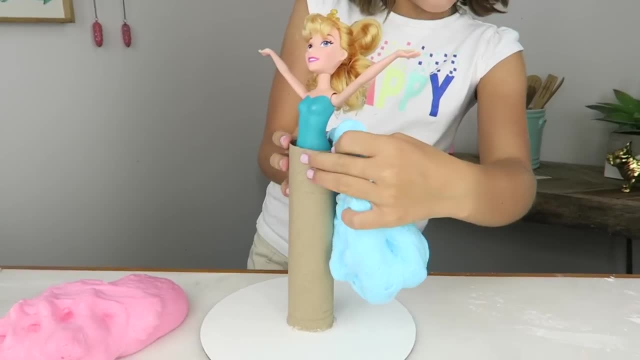 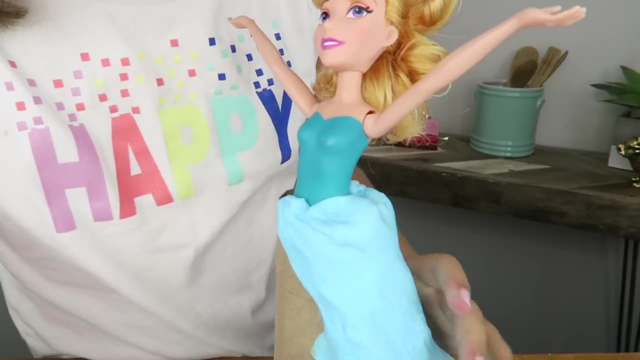 So this is what we're going to do. We're going to get the slime in there. I'm going to hook it right against her waist and kind of push it down into the paper towel tube And then kind of let it droop down. 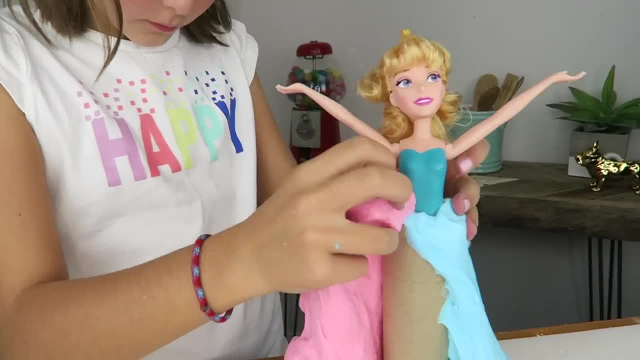 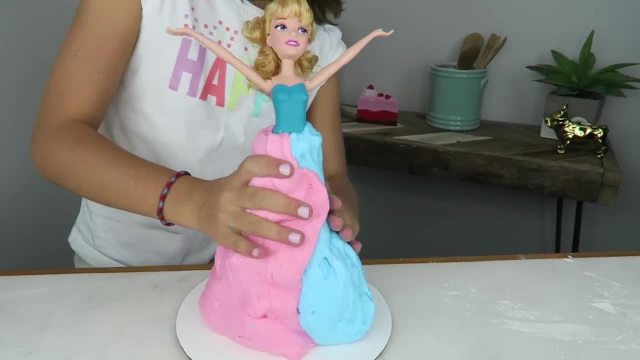 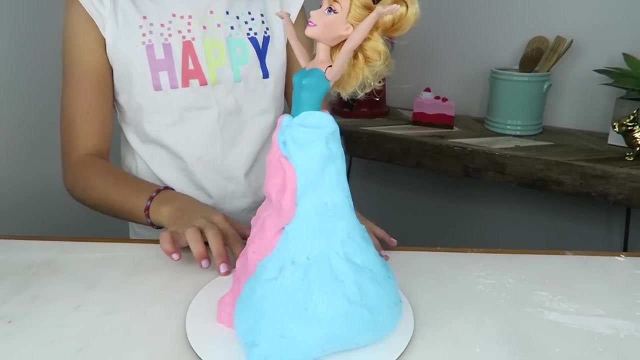 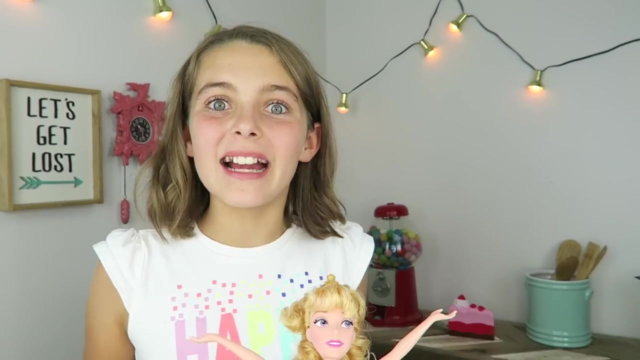 All right time for side pink. Okay, you can kind of form it in any way you want to. Oh yeah, This reminds me. Reminds me of like ice cream or cotton candy Slime dress. Let's put some rhinestones on it. 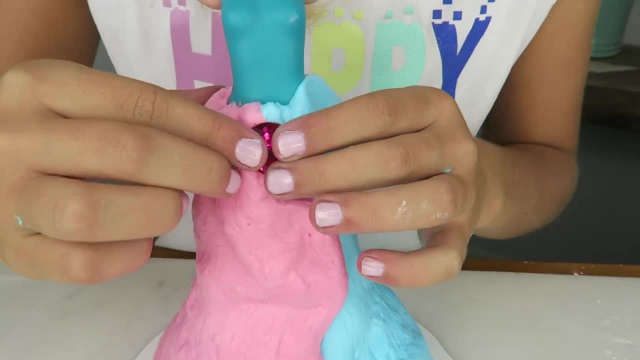 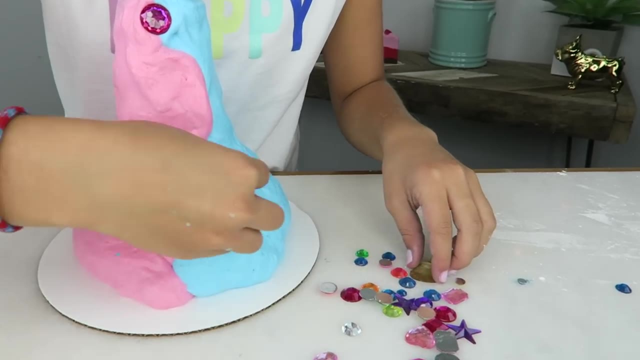 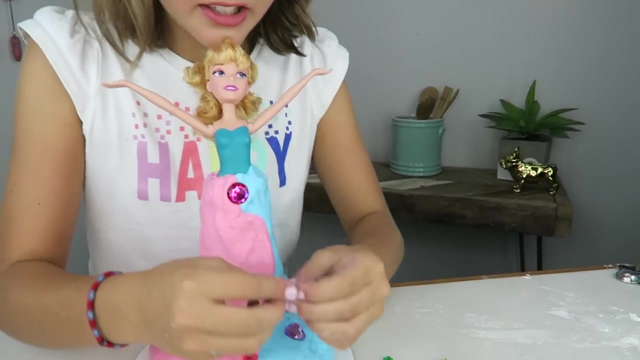 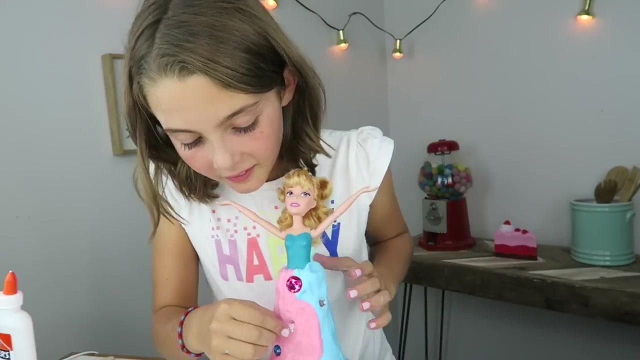 So I'm going to put this one right there, Okay, And then I'm going to put just a whole bunch of these all around her dress. Wow, they're sticking really good. Oh my gosh, Look at all these amazing colors. 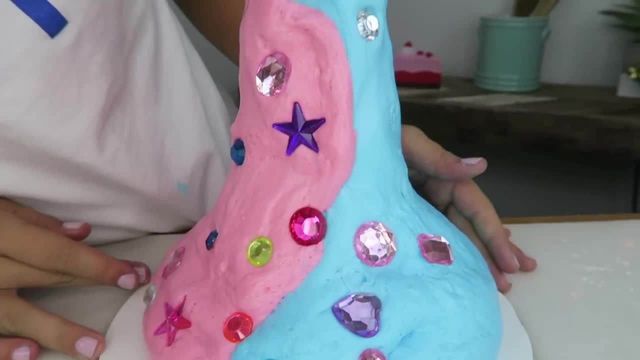 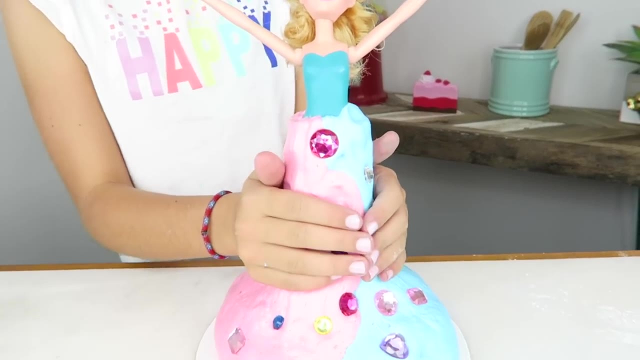 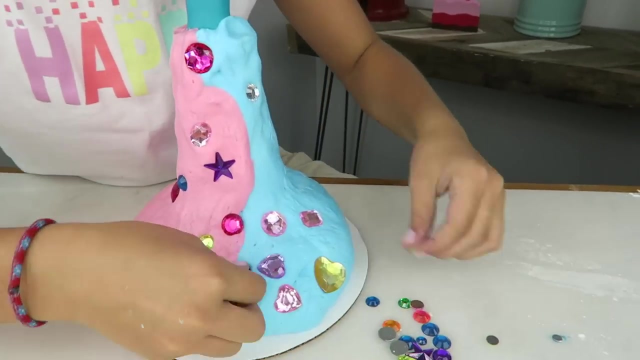 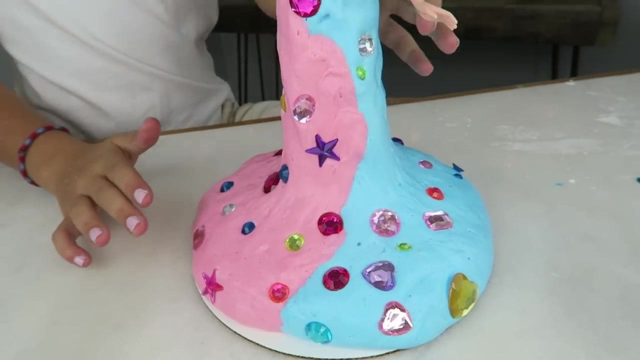 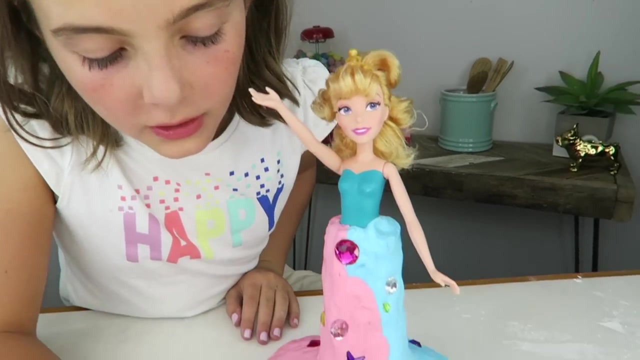 This kind of reminds me of like a mermaid dress, where it's like: stick right here and then it poofs out at the bottom. Let's put some rhinestones all around. oh my gosh, I love the colors, how it like smooshed together and like formed like. 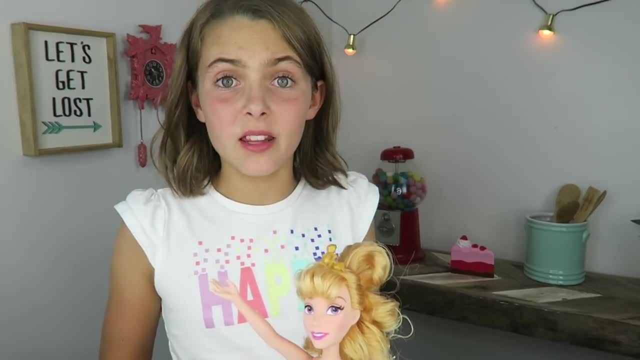 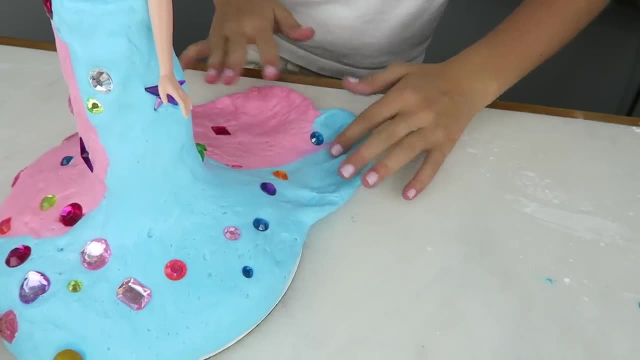 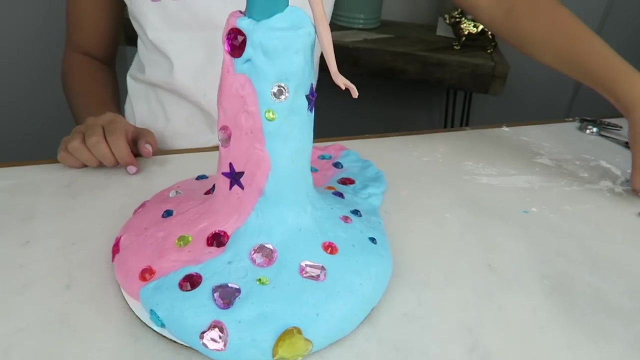 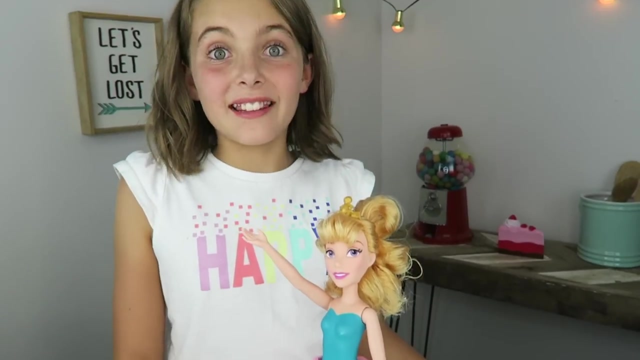 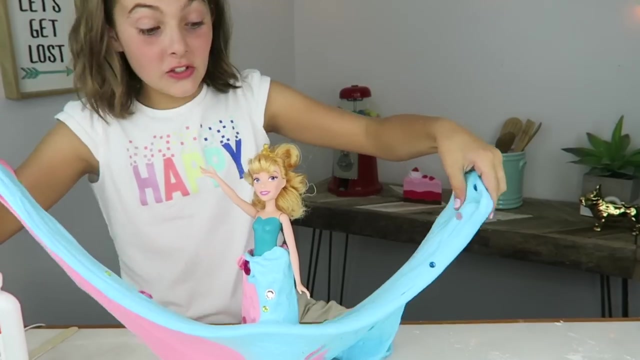 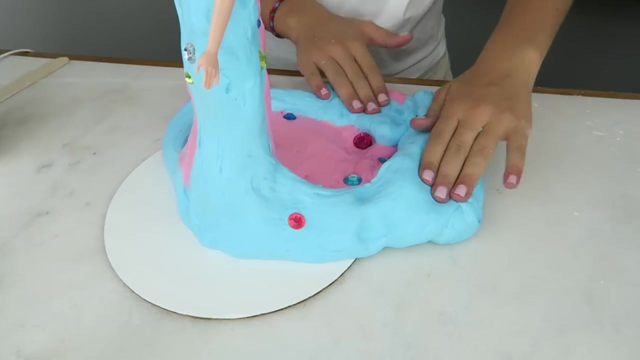 one a slime. let's give her a train in the back, pull it back just like this. so mix like a little train in the back, a little caboose. okay, let's try a new style. here's one idea: this is a really big dress there, just like that giant train in the back. 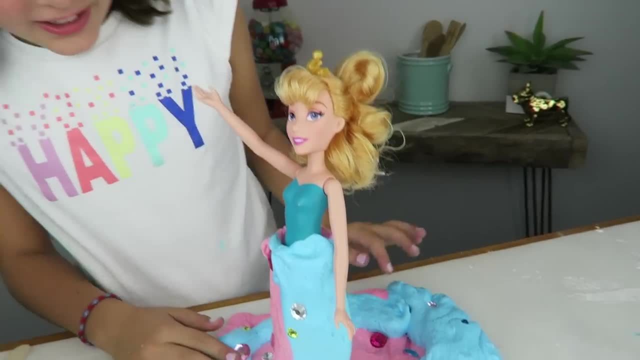 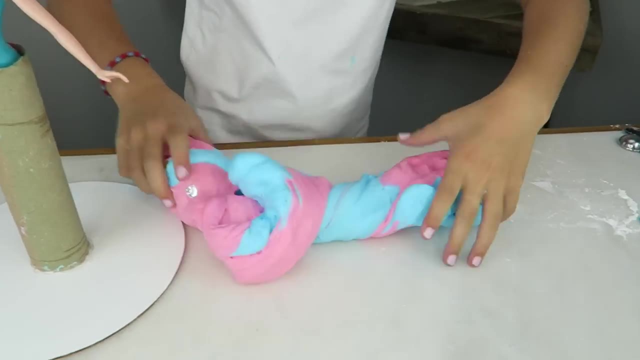 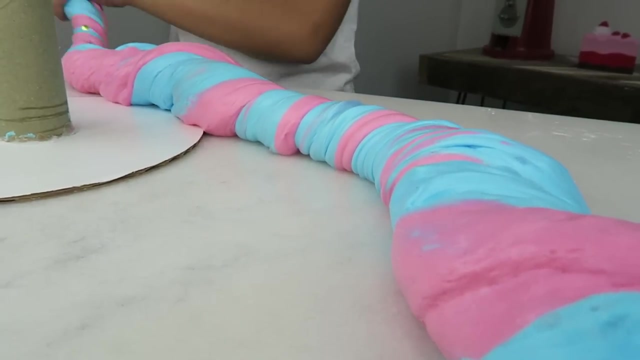 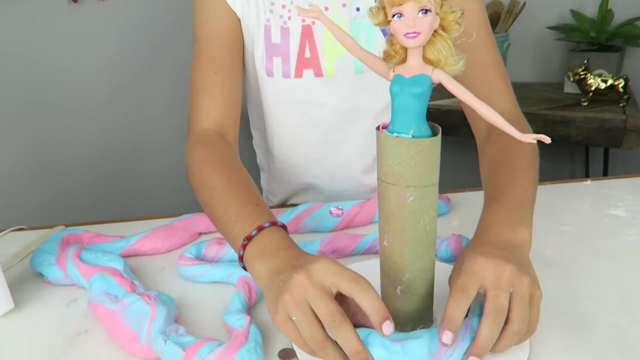 okay, new style. okay, let's twist these two colors together. twist it like taffy. you can lay down if you want. makes it kind of easier. you can twist it as much as you want. so I'm just going to spiral around her dress, starting at the bottom. 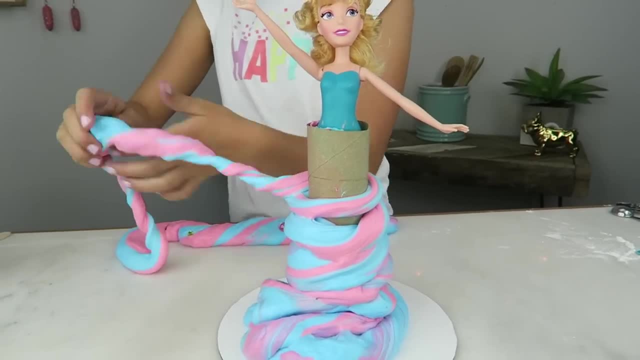 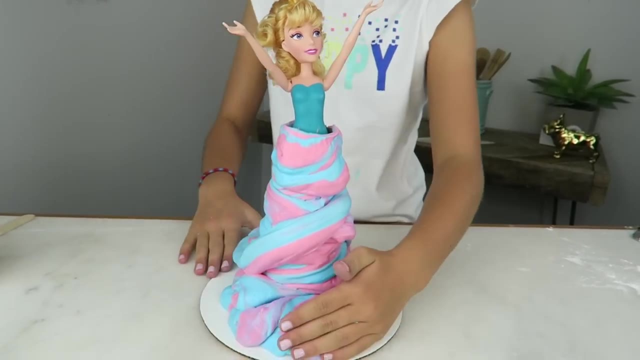 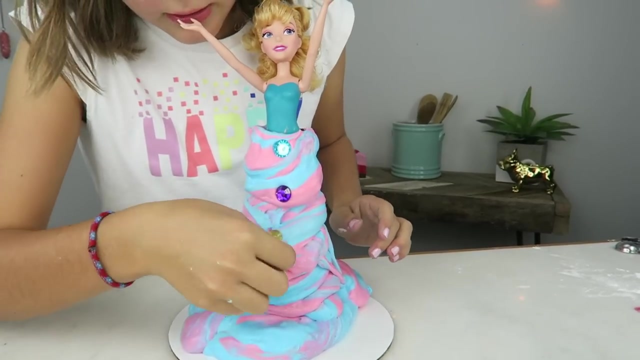 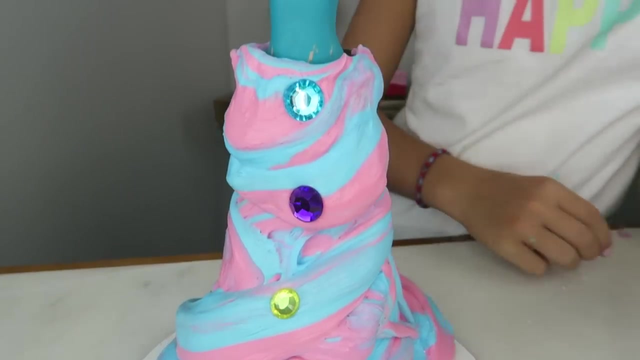 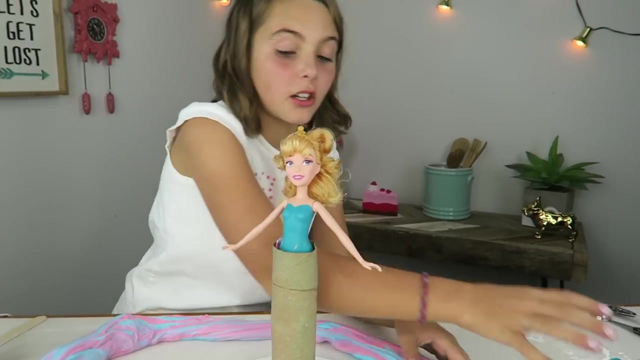 time for some more rhinestones. how does that look? does it look pretty? okay? let's try one more fashion style. this time I'm going to start from the top and go to the bottom, alright, so I'm just going to put it up on our shoulders and cross. 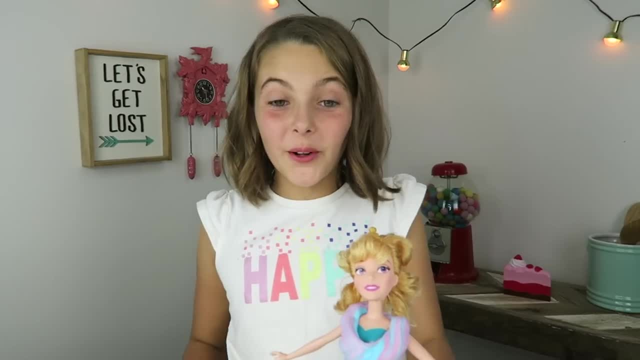 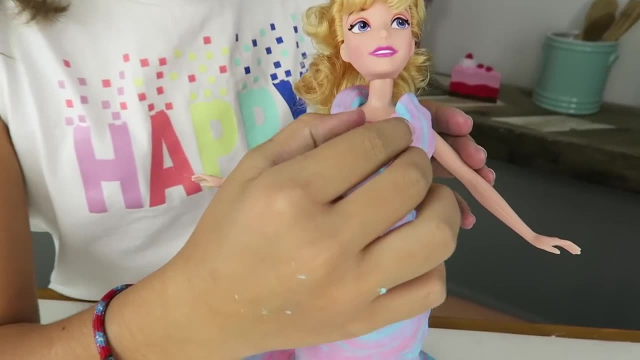 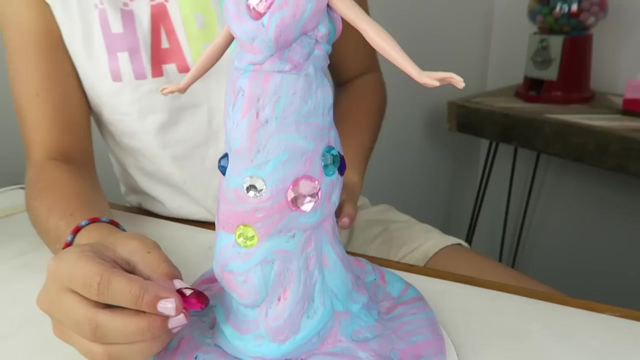 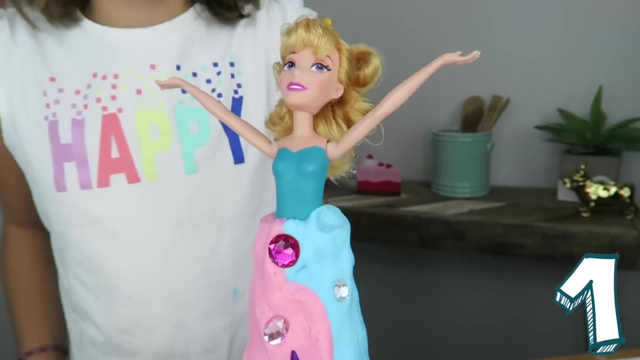 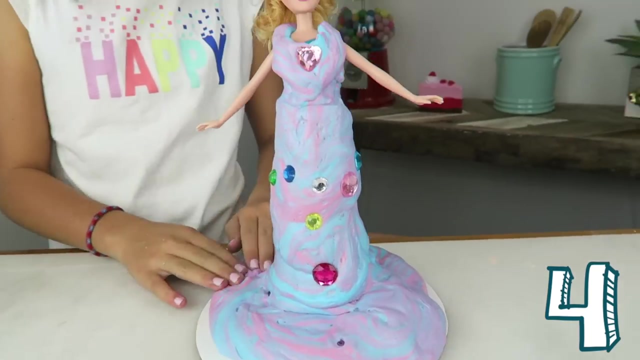 our blue and pink became purple. whoa, now we have three different colors. I'm just going to put a heart right there. which one's your favorite style? one style to style three, or style for comment down below. you can also use the slime on the little dolls. see, check this out, you can check. 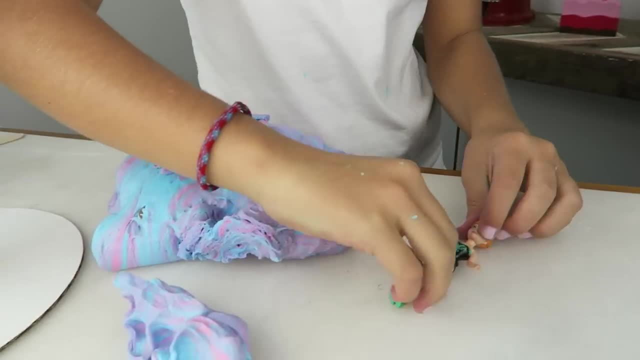 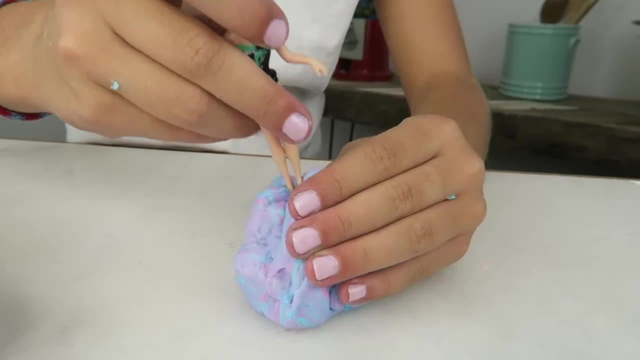 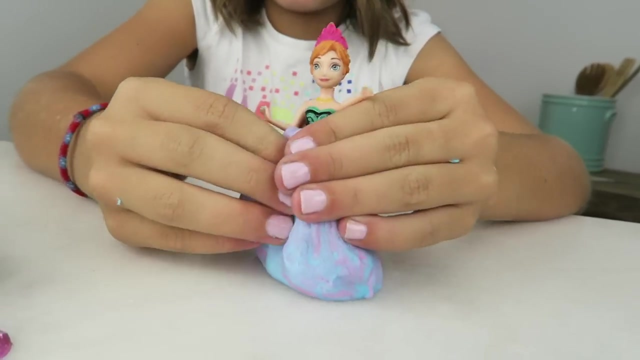 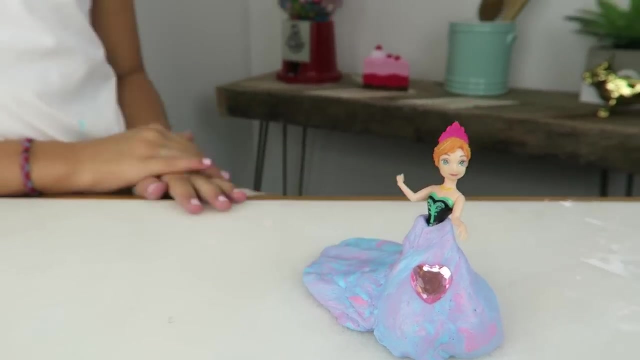 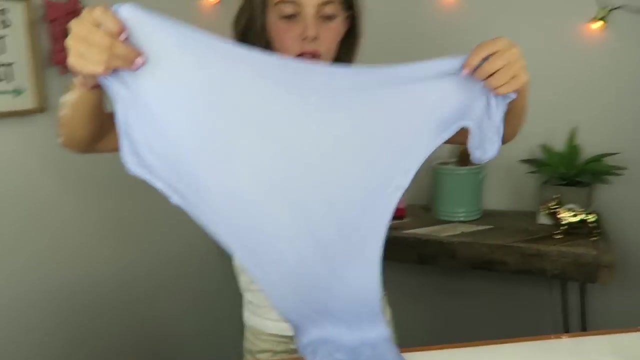 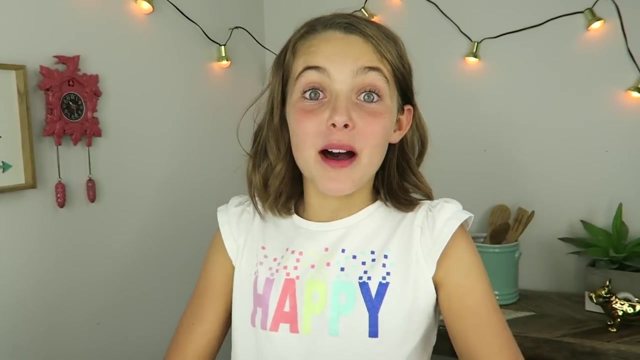 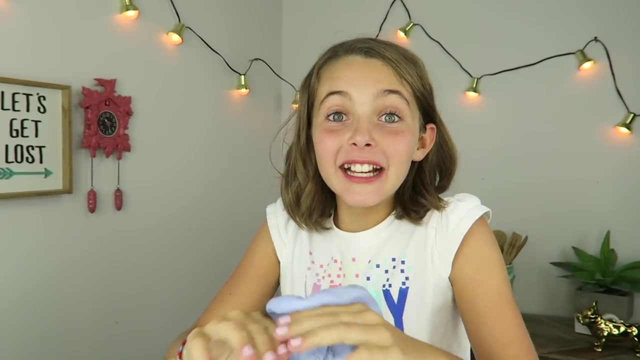 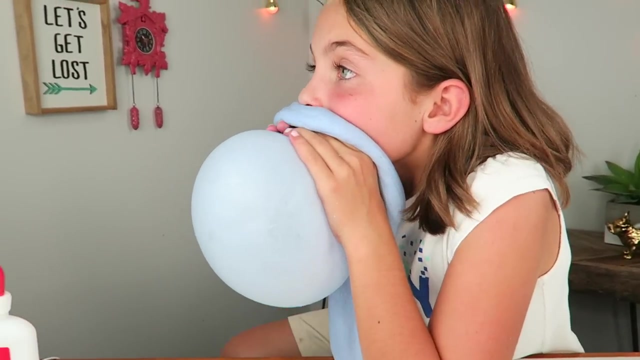 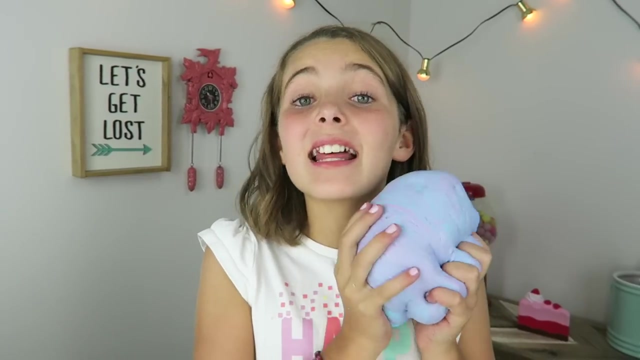 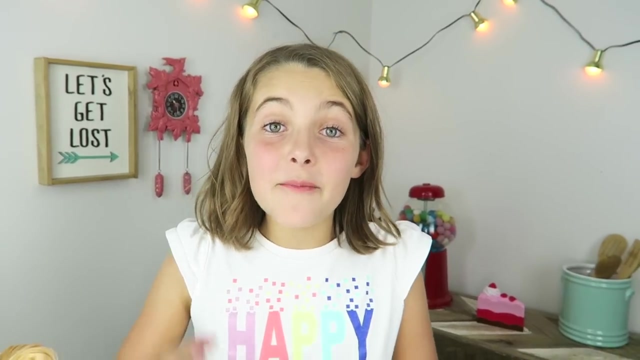 out. you can just take a little little piece and then make it into a dress and then stab her into it. yeah, yeah, yeah, yeah, and don't forget to like, subscribe and comment down below which fluffy, slime princess dress was your favorite. see you guys next time. bye.